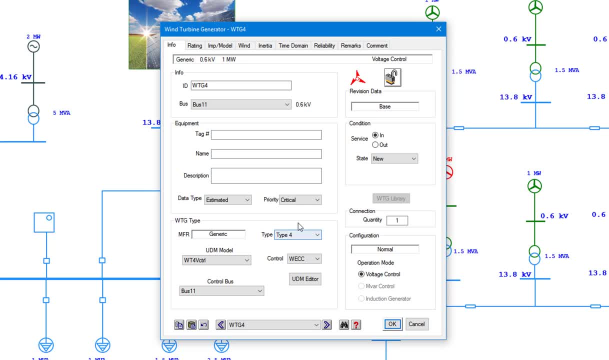 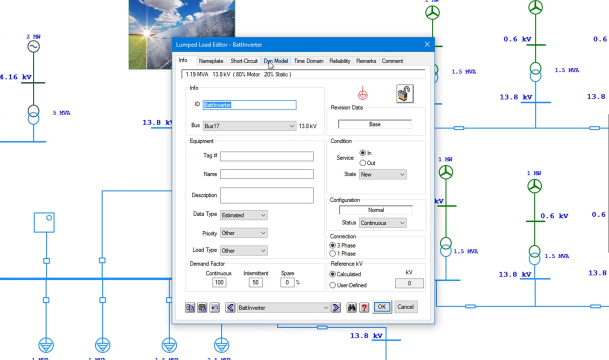 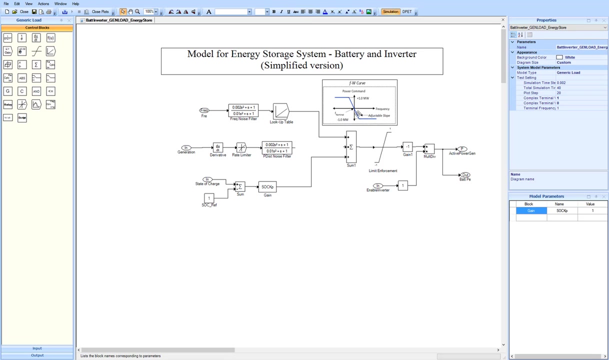 the technology type. the program also provides you the capability to specify the impedance, inertia, as well as other dynamic details for the wind turbine generator. etab allows you to model dynamic models for energy storage devices as well. the energy storage device modeling can be simply accomplished using etab udm editor. here's an example of a model for energy storage system, including the battery. 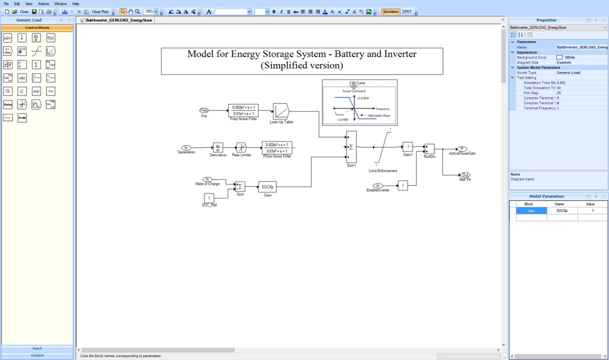 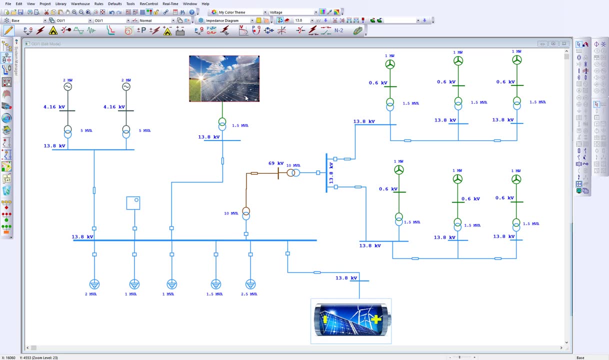 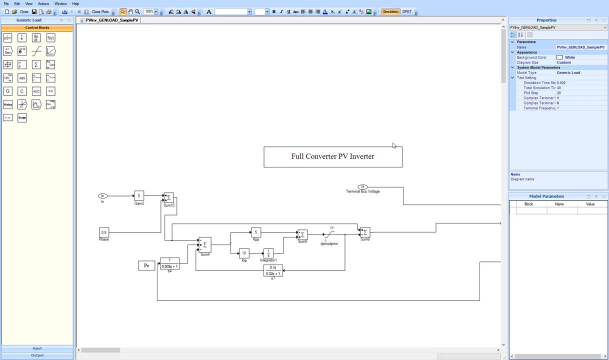 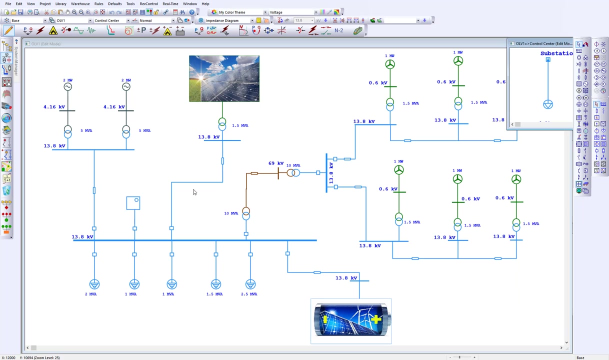 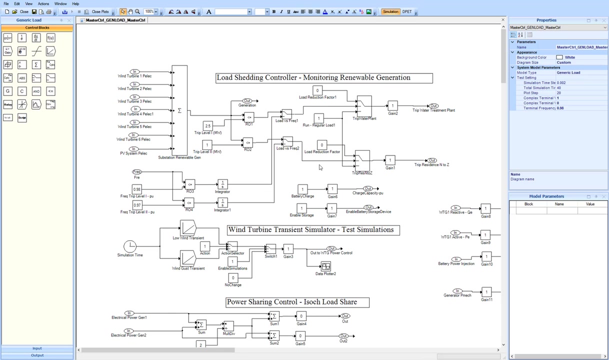 and inverter using a conventional frequency power curve. you can also define the dynamic model of the pv inverter, once again by utilizing etab udm editor. etab also allows you to model secondary controllers, such as a microgrid controller. the microgrid controller allows you to include inputs from various UDMs, such as wind turbine. 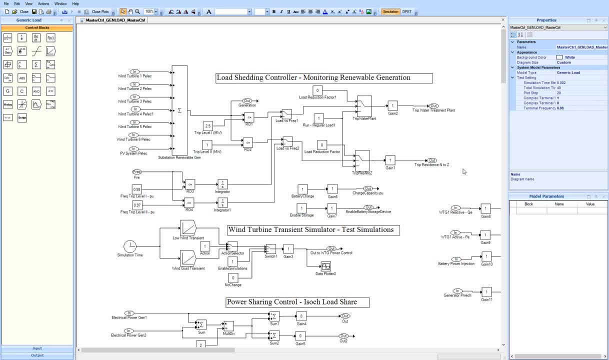 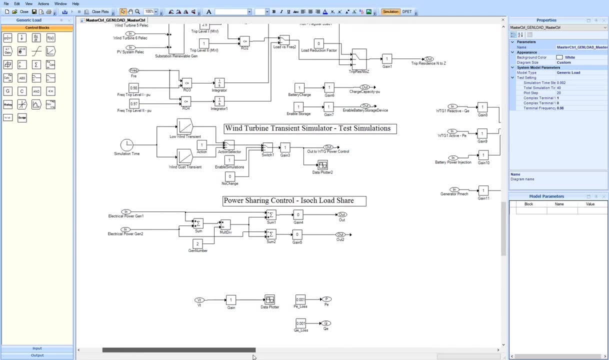 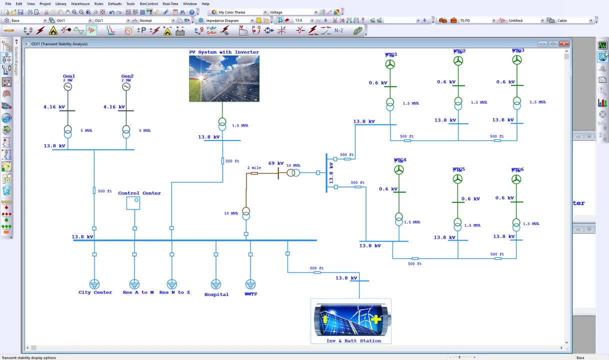 and PV system energy storage device, and also define various complex logics such as load shedding, power sharing and other types of microgrid functions. in order to run a dynamic simulation, simply switch over to transient stability and click on the run transient stability button once the transient stability calculation is. 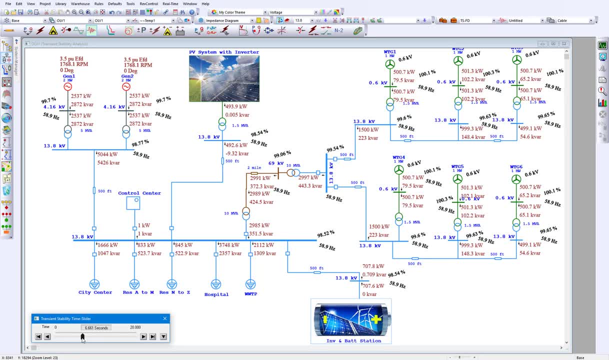 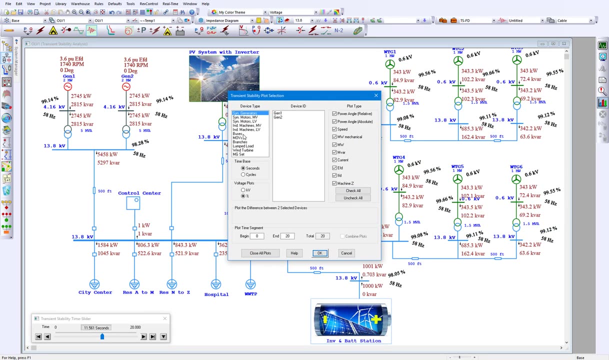 completed. you can simply move the time Slider and see the effect of the analysis, such as change in voltage, frequency and power in the network, directly on the one-line diagram. you can also see the same information with the help of plots. simply select the component type and the type of chart you. 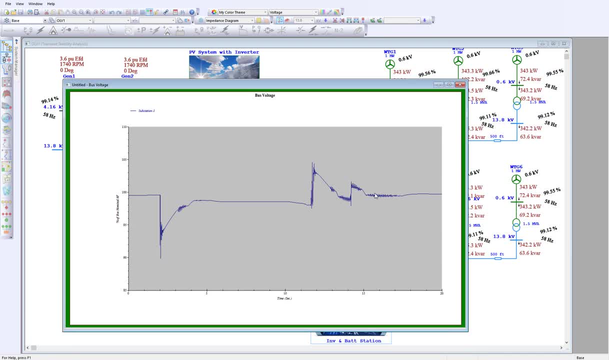 would like to plot, and then the program essentially gives you the information directly. here we can see the microgrid controller trying to compensate and correct its total logics rate. the diagram below shows aай sending your sense of the table. wonderful, that's a great idea. add the information that working. 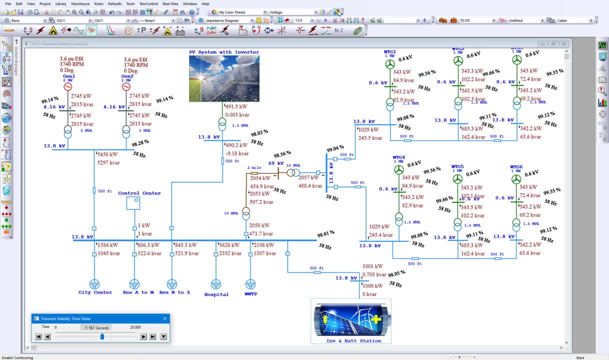 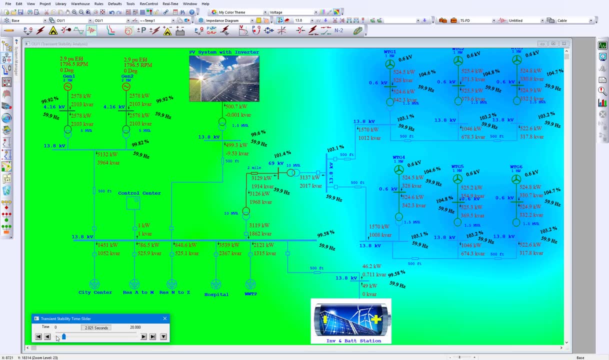 the load impact in the system. you can also turn on color contouring and simply step through various time steps and see the impact of the load impact in the system. here we can see the load was added and then we can go through the power swing and see how the system is trying.